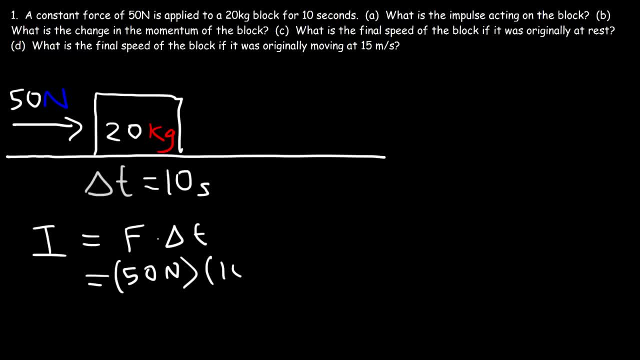 50 Newtons acting on the block for a time of 10 seconds. So 50 times 10 is 500.. So it's 500 Newtons times seconds. So that's the impulse acting on the block. Now you might use a different symbol for impulse, but in physics just be careful with the. 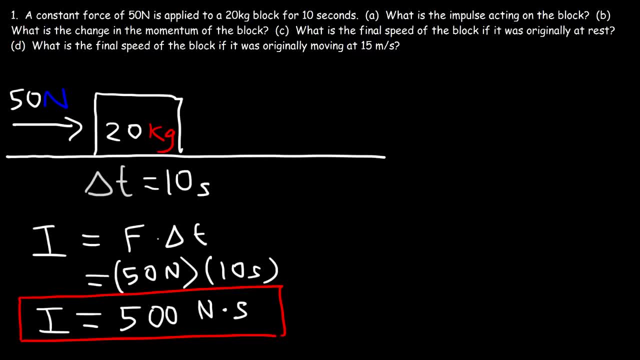 letter I In this video I'm using it as impulse. In another chapter it could be represented as inertia or sometimes in other chapters, intensity, So just be careful with that. So you need to know the context in which that letter is being. 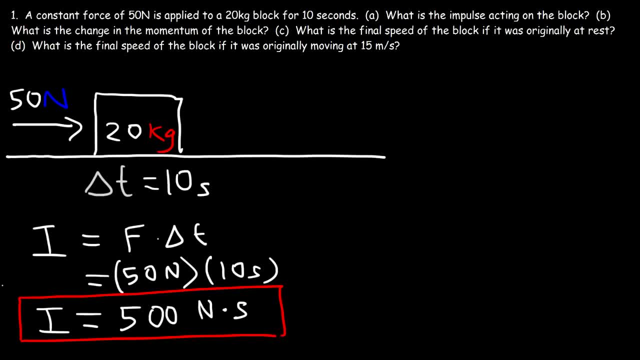 used. Now, what is the change in the force acting on the block? So we know that force acting on the block is the change in momentum. Impulse is equal to the change in momentum, So the change in momentum is going to be positive: 500 Newtons times, seconds, or kilograms times. 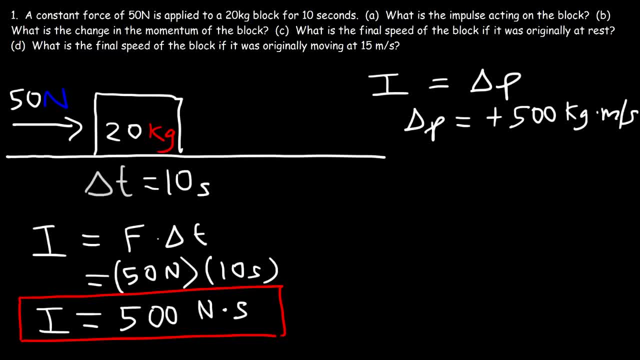 meters per second, because momentum is mass times. velocity Mass has the units kilograms. velocity is in meters per second, So it's important to know that a Newton times a second is equal to a kilogram times a meter per second. Part C: What is the final speed of the block if it was originally at rest? The? 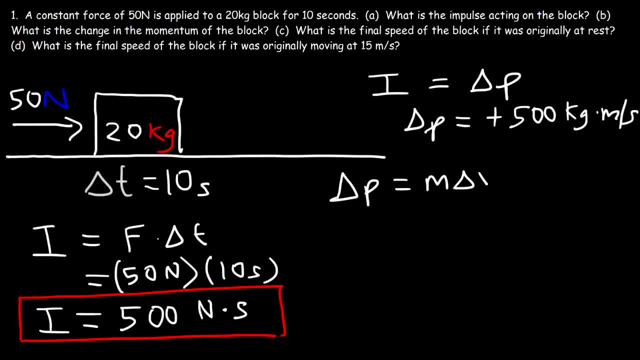 change in momentum is equal to mass times the change in velocity, So that's mass times, the V final minus the V initial, So the change in momentum is 500.. The mass of the block is 20.. We're looking for the final speed. 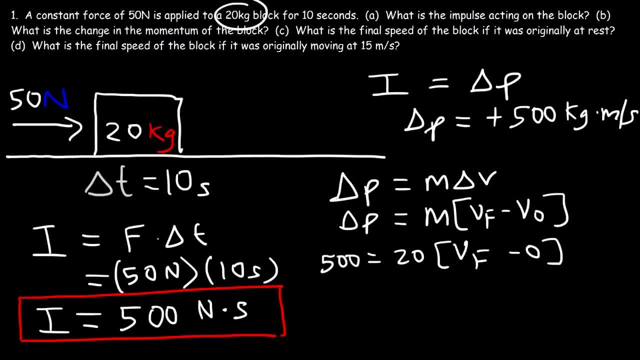 and the initial speed is zero. So 500 divided by 20 will give us a change in velocity of 25.. So therefore, the final speed for Part C is 25 meters per second. Now let's move on to Part D. What is the final speed of the block if it was originally moving at 15 meters? 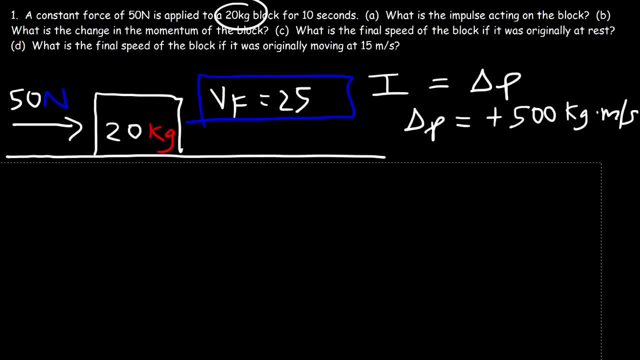 per second. So let's make some space because there's a lot of stuff on this page. So we're going to use the same example. In this equation, delta P is equal to M delta V, where the change in velocity is V final minus V initial, So the change in momentum is positive 500.. The mass is 20.. We're looking. 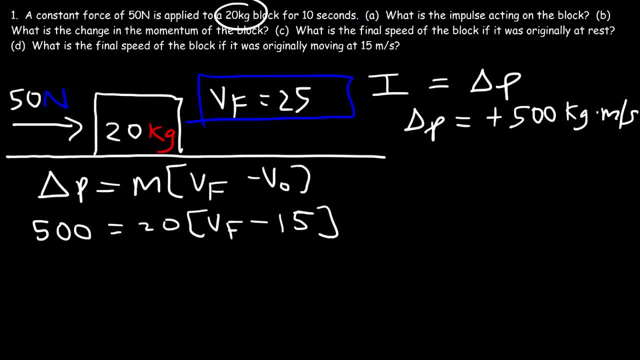 for the final speed, but the initial speed this time is 15.. So 500 divided by 20 is still 25.. So the change in velocity is 25.. So if we add 15 to both sides, the final speed will be 40.. 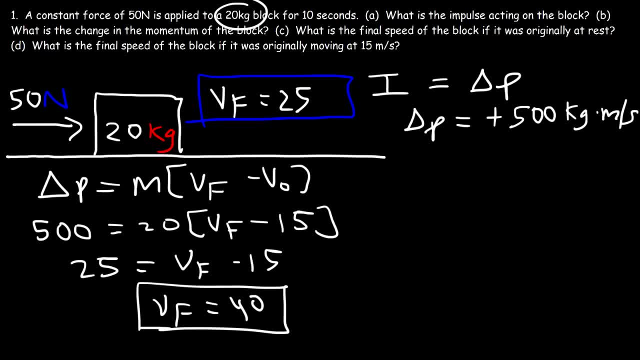 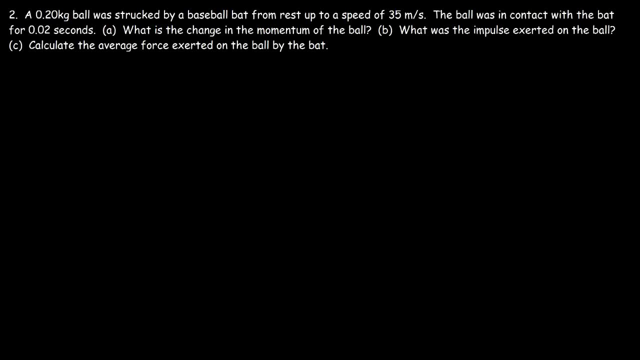 So if the initial speed was 50, the final speed would be 75.. If the initial speed was 100, the final speed would be 125.. The change in velocity is going to be the same because we're dealing with the same force acting over the same time. 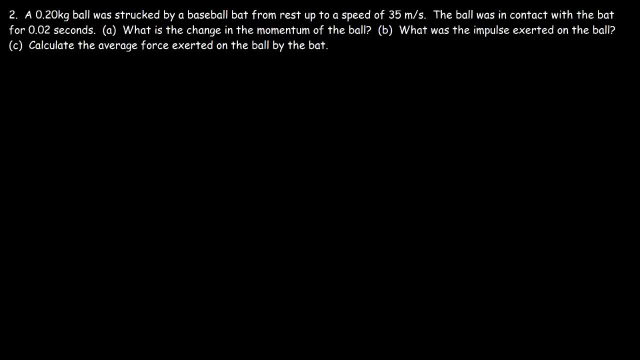 Now let's move on to number two. A point 20 kilogram ball was struck by a baseball bat from rest up to a speed of 35 meters per second. Now the ball was in contact with the bat from only 0.02 seconds, which is 20 milliseconds. What is the change in the? 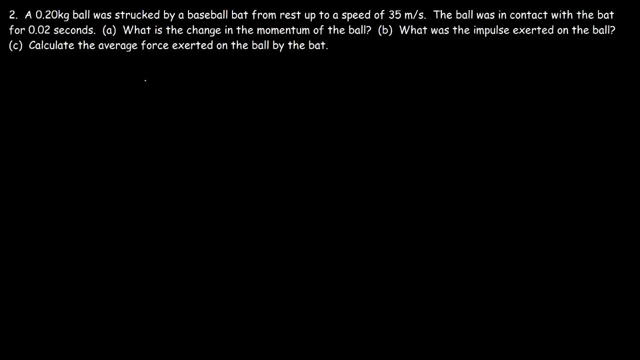 momentum of the ball. So the change in momentum is equal to mass times the change in velocity. So that's going to be M times V final minus V initial. So the mass of the ball is 0.20 kilograms, the final speed is 35, and the initial speed 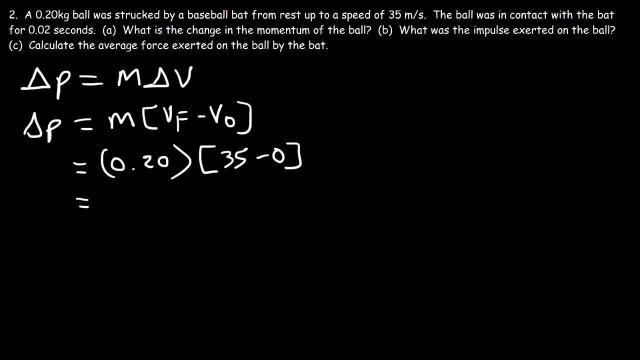 is 0. So it's 0.20 times 35.. So the change in momentum is 7 kilograms times meters per second. So that's the answer to Part A. Now what about Part B? What was the impulse of the ball? 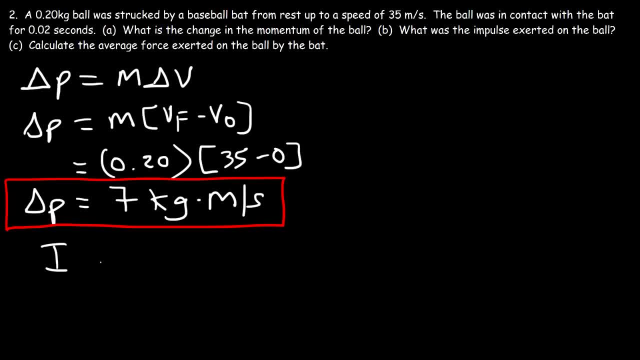 What was the impulse exerted on the ball? Now, impulse is equal to the change in momentum, So the impulse is going to be positive 7 Newtons times seconds. If the impulse is positive, the ball is speeding up. If the impulse is negative, the ball 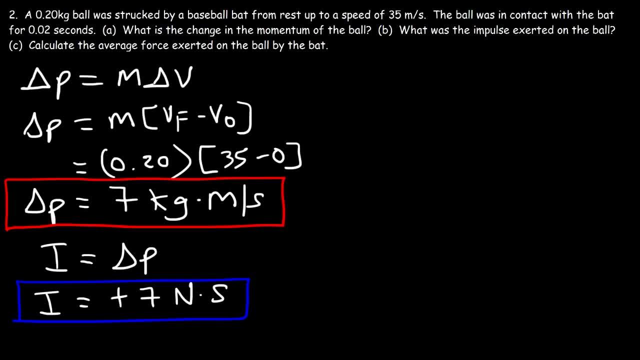 will be slowing down. Now let's move on to Part C: Calculate the average force exerted on the ball by the bat. So let's say this is the bat and it strikes the ball, So the bat is going to exert a force on a. 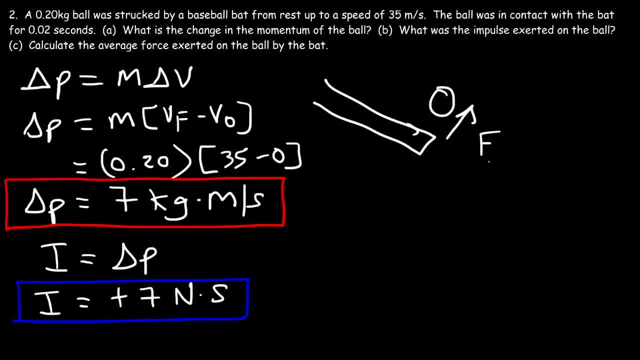 ball. We need to calculate that average force exerted by the bat on the ball. So how can we do so? So recall that impulse is equal to force multiplied by the change in time, The impulse is positive. 7. We're looking for F and the contact time, the time that the bat is in contact with the ball. 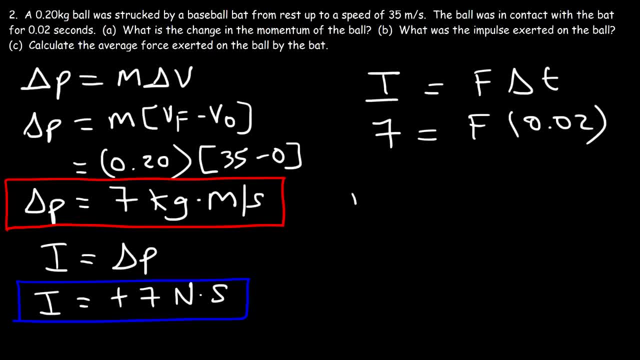 is 0.02 seconds. So the average force is going to be 7 divided by 0.02 seconds, And 7 is associated with the units Newtons times seconds divided by 0.02 seconds. So we can see that these units will cancel. So 7 divided by 0.02 is 350.. So the 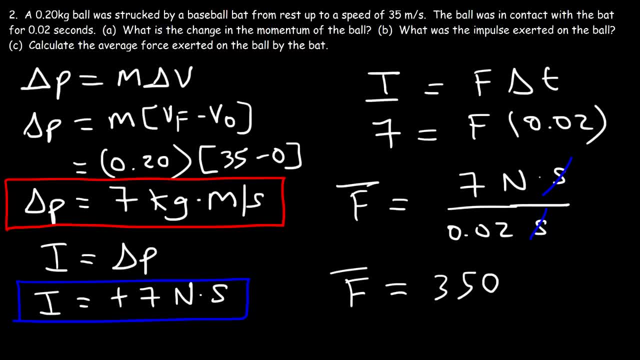 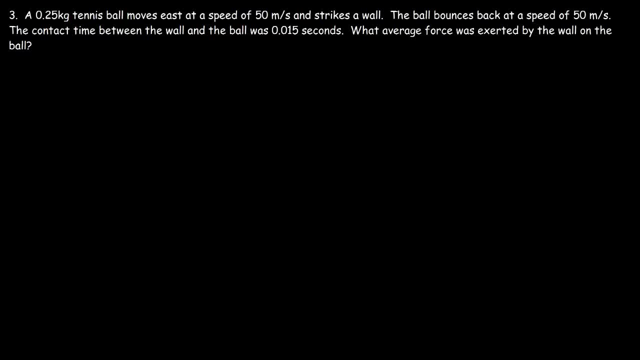 average force exerted on the ball is 350 Newtons, And so that's it for this problem. Number three: a 0.25 kilogram tennis ball moves east at a speed of 50 meters per second and strikes a wall. So let's say: this is the wall, and here is. 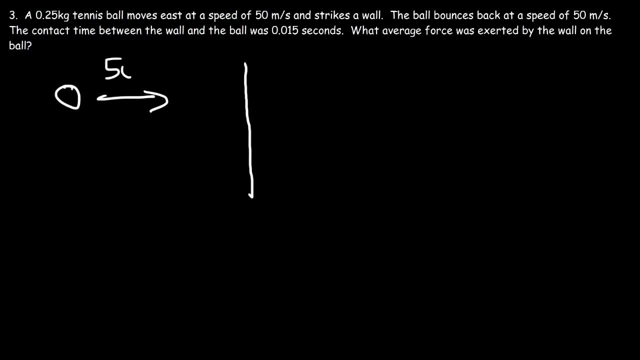 the ball moving east at a speed of 50 meters per second. The ball bounces back at a speed of 50 meters per second, So it's going to go back this way. The contact time between the wall and the ball was 0.015 seconds. 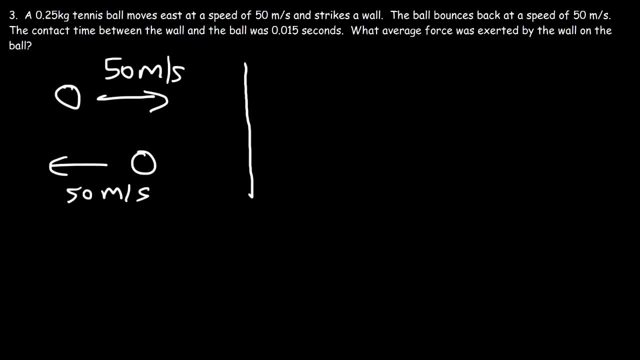 What average force was exerted by the wall on the ball? Now, when dealing with momentum, you need to deal with velocity. Momentum is mass times velocity, not mass times speed. So momentum is a vector. The velocity of the ball is positive 50 because it's. 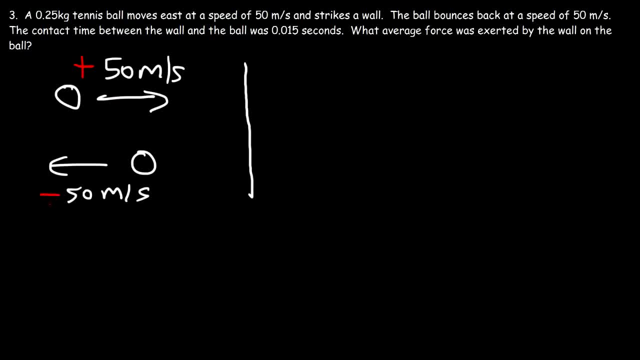 going east. Once it strikes the wall, the velocity is negative 50 because it's going west, And so the wall exerted a force that was directed west because it caused the object to travel in the westward direction. So we should expect that this force should be negative. So what equation can we use to calculate?